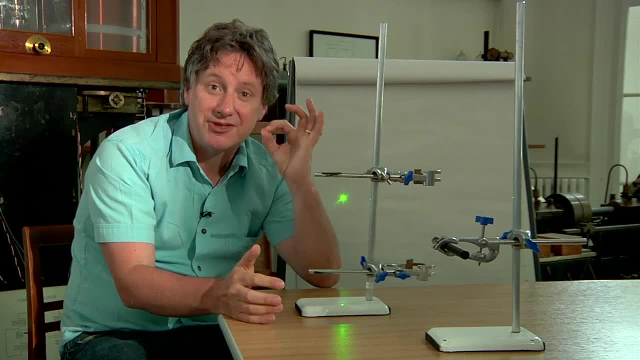 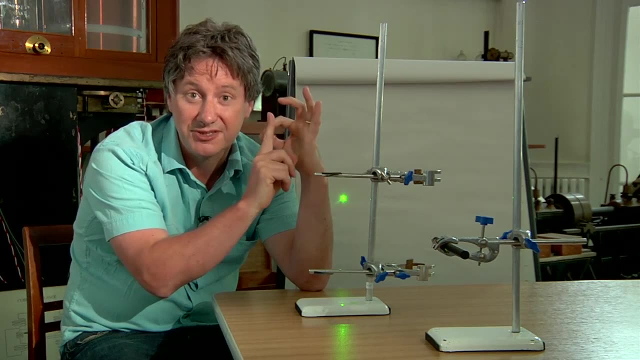 And normally and perfectly reasonably, they tell me, they'd expect the spot to be obscured by the shadow of the wire. So if this is the spot, they'd expect the wire to move in front of it, something like that, So that on the screen we'd see a dark line down the centre. 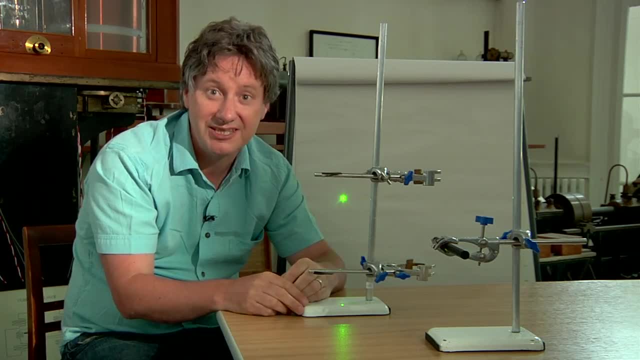 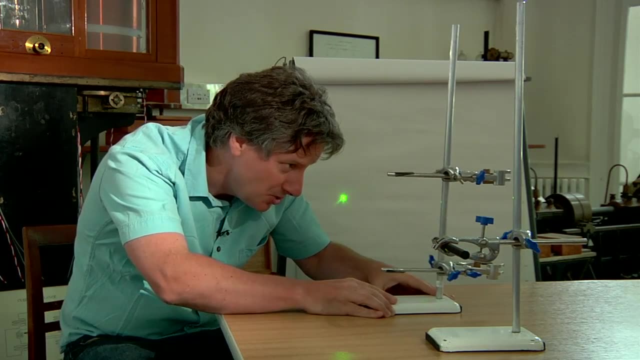 of the spot, But in fact that's not what we see. Let's take a look at what actually happens. So I'm going to slide the wire across And you need to be quite careful to get it. There we go. You should just be able to see. 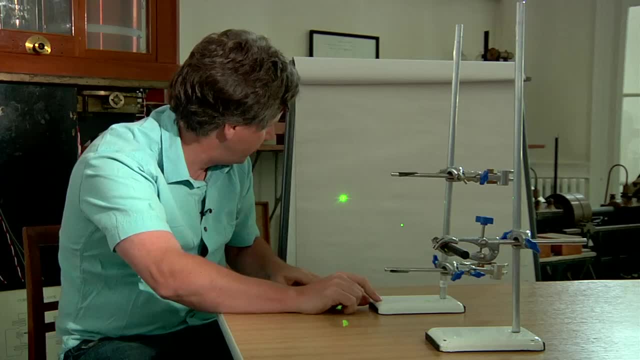 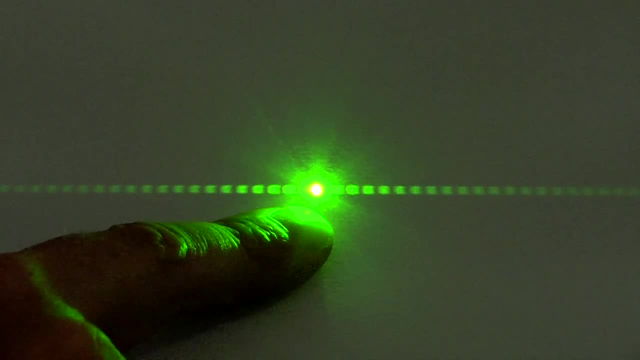 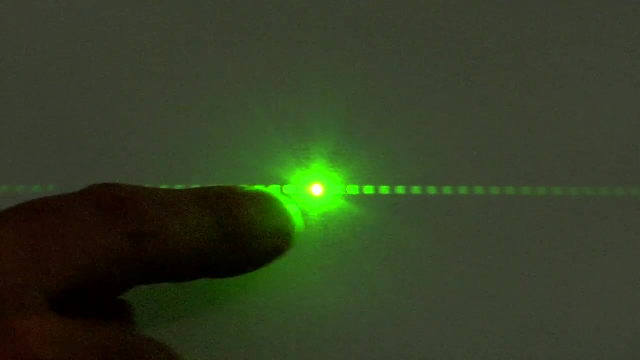 here where the laser is shining over the wire And on the screen. oh wow, If you look at the spot, you should be able to see that there's no dark line down it at all. It's still perfectly bright, But on either side of it you can see bright and dark bands extending out many. 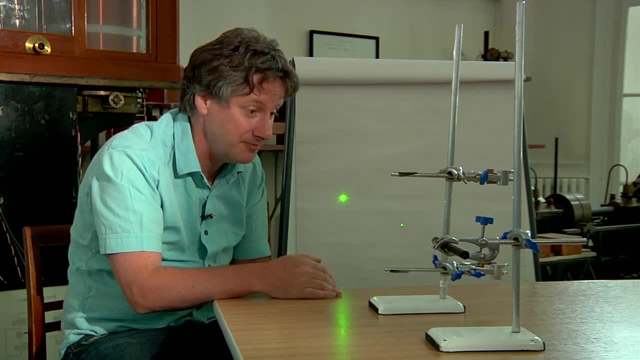 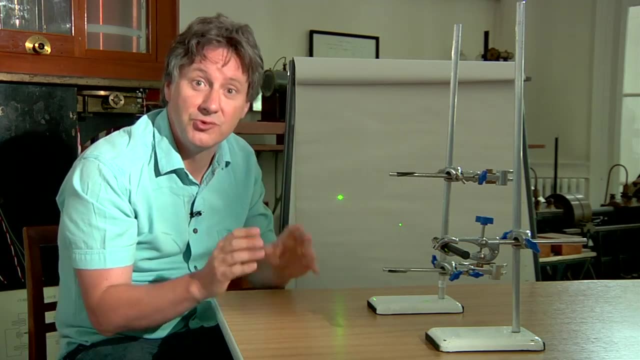 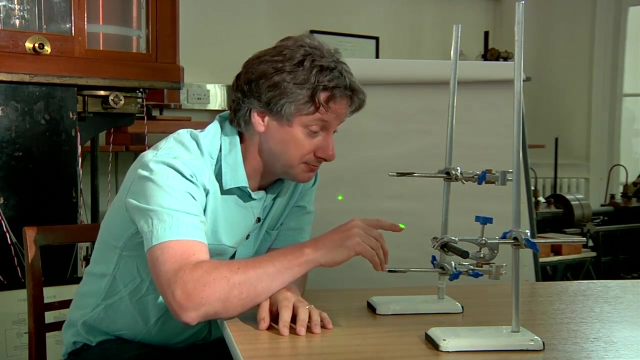 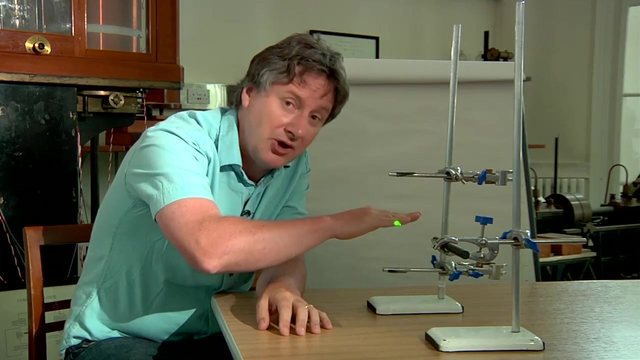 times the diameter of the wire or the laser beam. So the question is: how do you relate this pattern to the wave nature of light? Well, light waves travel from the laser over to the wire and they diffract around each side of the wire, That is, they're bent to fill the space beyond and behind the wire, extending 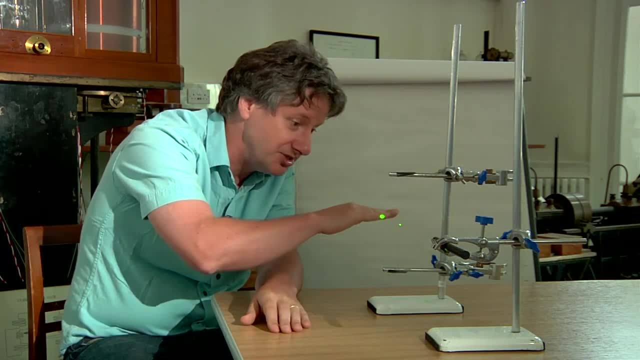 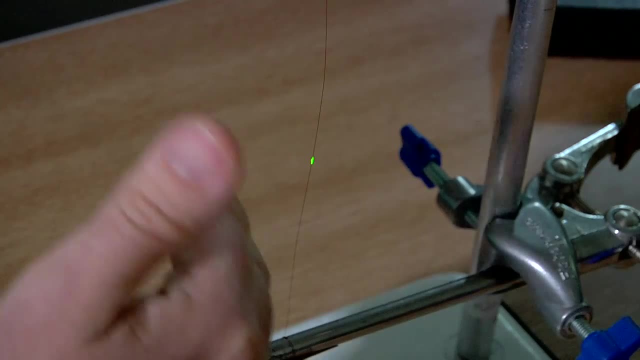 over to the screen. So in this region we observe interference between the light and the laser beam And it goes up to a certain point down the line in a 16 degree angle. So as the laser beam goes up, the light goes down to the center of the wire And there's no light going around. 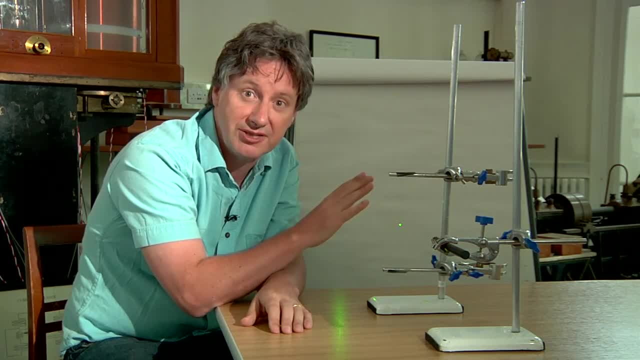 it. So we observe the interference between the light waves that have come round one side of the wire and around the other, Where the waves are in phase, that is, where the crest of one wave matches the crest of a wave that's come around the other side of the wire. we 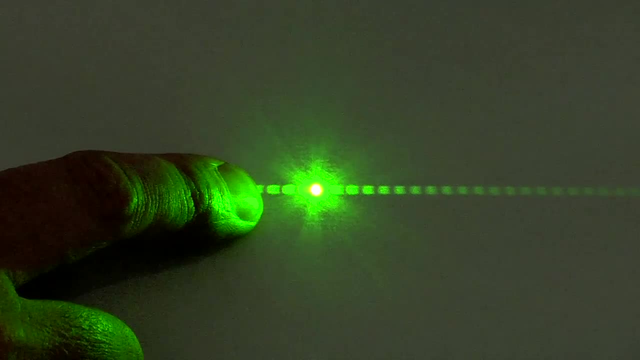 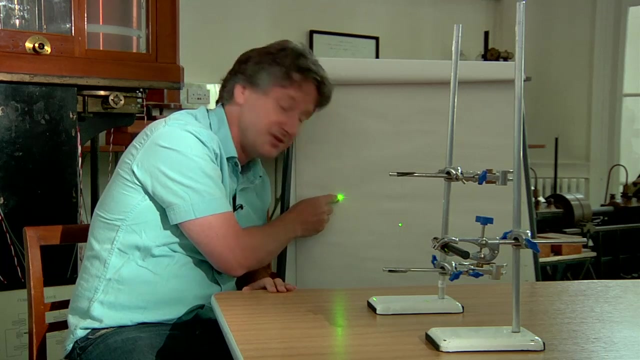 observe constructive interference And that's what leads to these bright regions on the screen And it's what explains the absence of a shadow in the center, In this region, each side of the wire, because this point is exactly equidistant from either side of the wire. 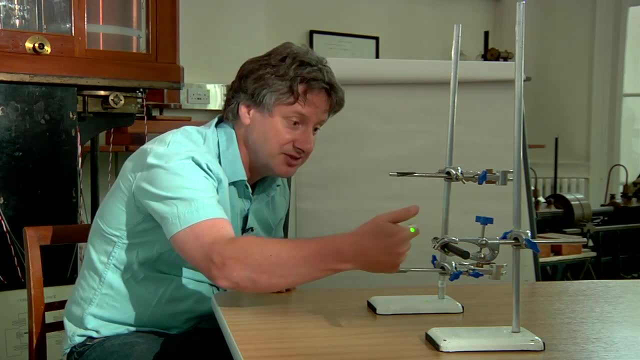 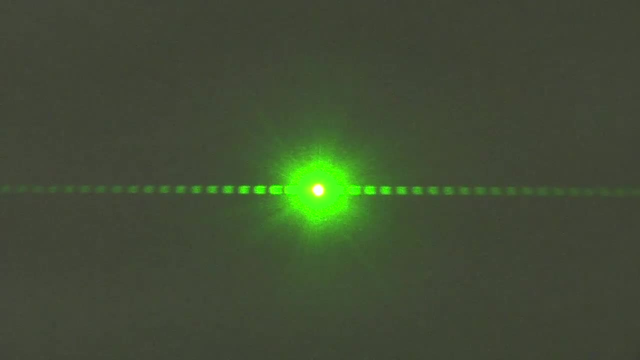 we also observe destructive interference. that's where the light traveling around one side of the wire interferes destructively with the white that's traveled around the other side of the wire, and that's what leads to the pattern we see on the screen now. it's easy to get lost in the